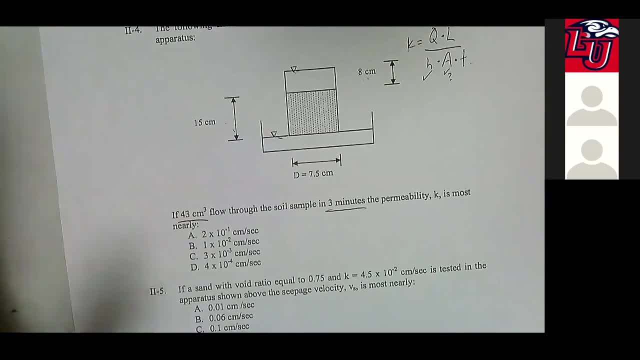 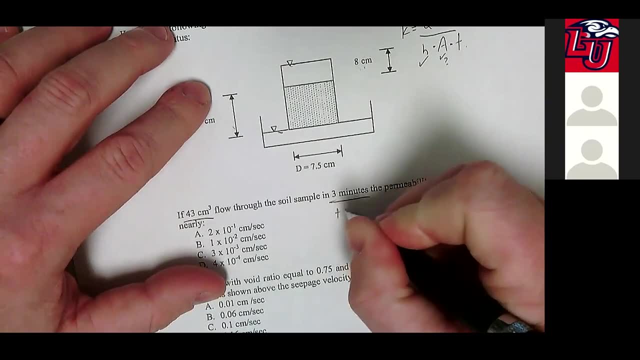 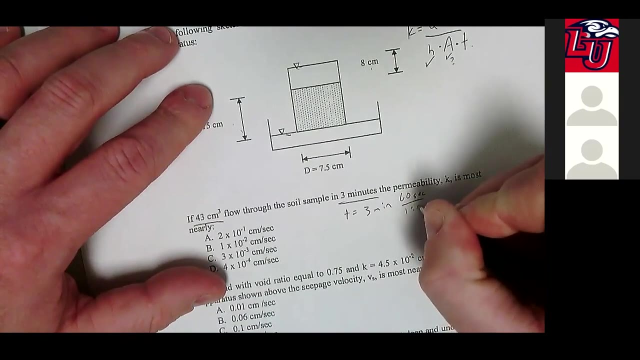 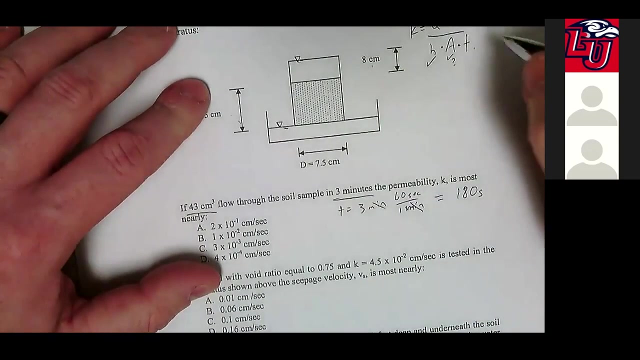 terms of seconds, but we can convert that, So let's go and do that now. So T is equal to three minutes times 60 seconds per one second minute. sorry for my sloppy handwriting, that's 180 seconds A we'll need to. 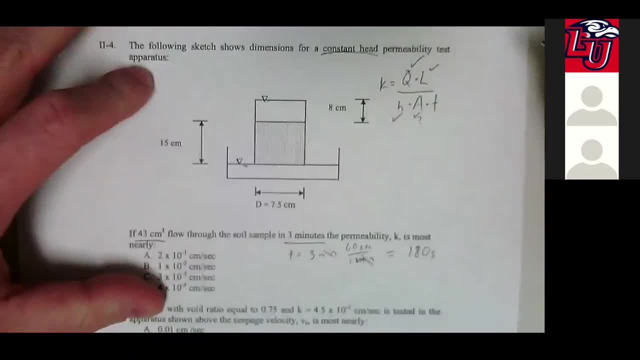 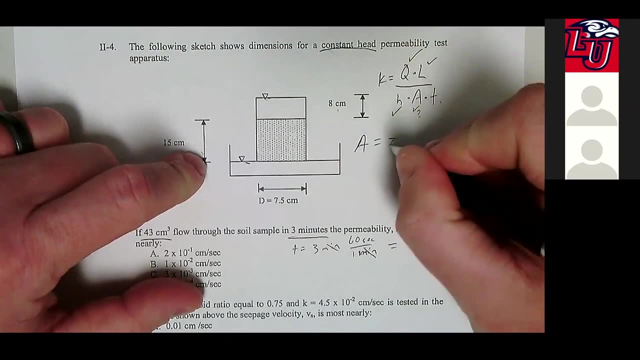 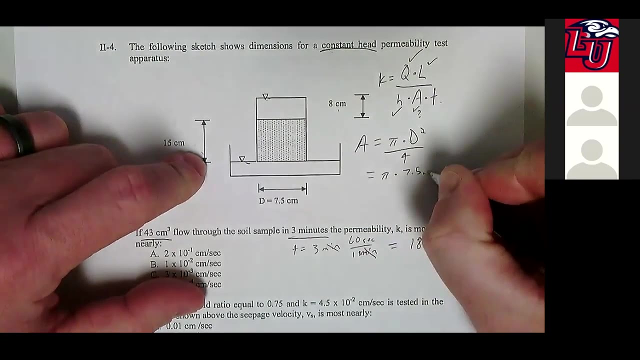 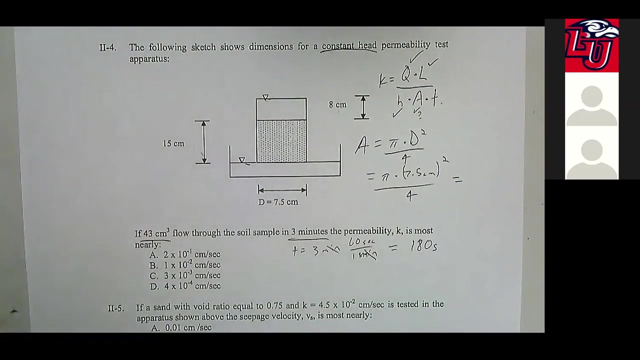 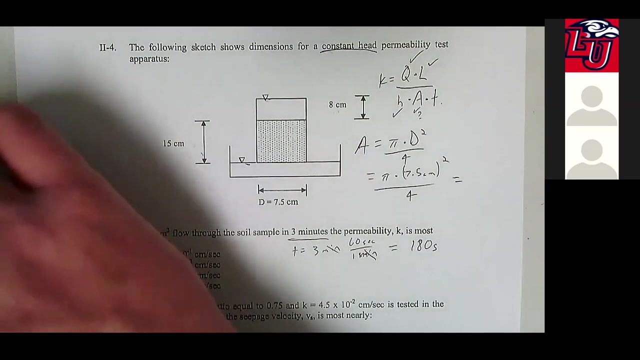 calculate to get cross-sectional area, So area of a circle, and that's pi D squared over 4.. That's pi times 7.5 centimeters squared divided by 4.. Again, I'm going to check my math here because I don't have my solutions handy- It's 44.2 centimeters. 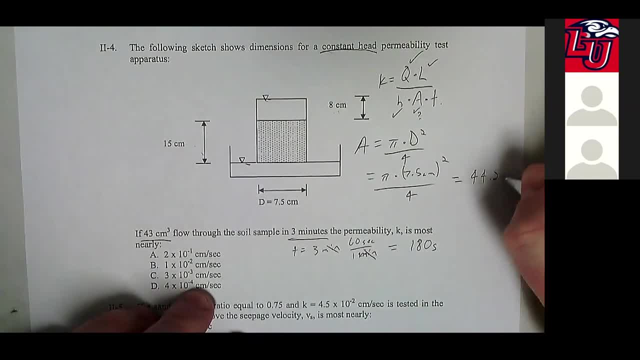 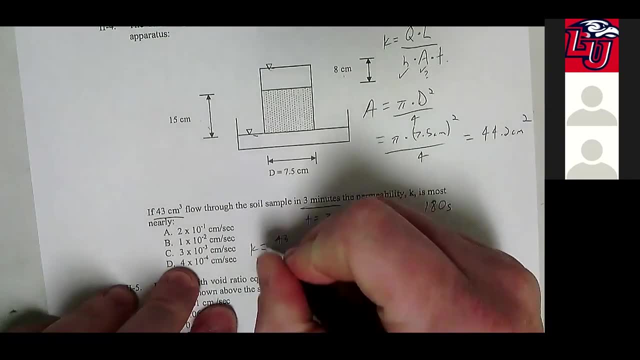 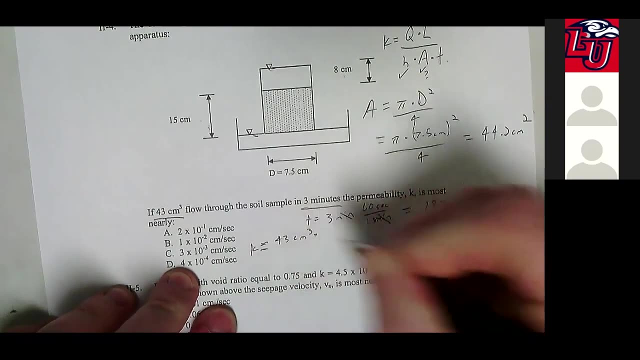 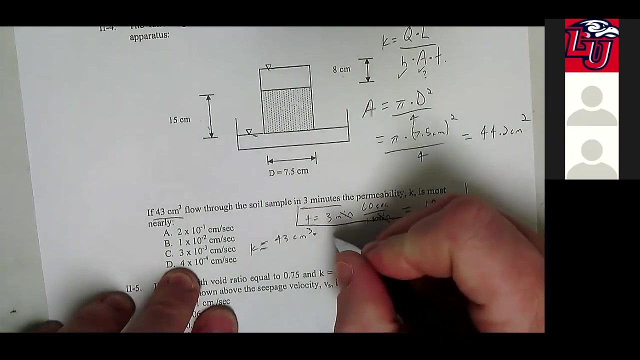 squared. So now we can just plug everything we've calculated back into the equation for k. So k is 43 centimeters cubed. That's the volume. I'll just try and box this out here so I don't get confused. Times L, which is 15 centimeters, divided by H, which is 23. 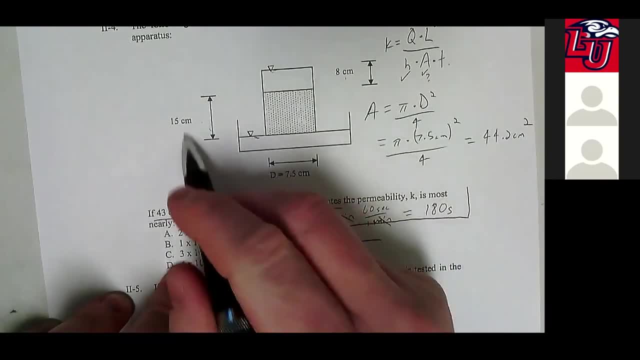 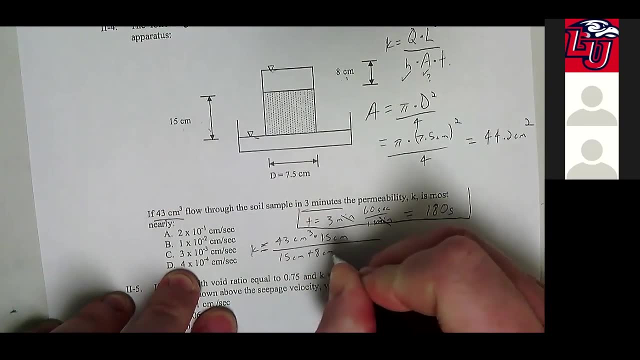 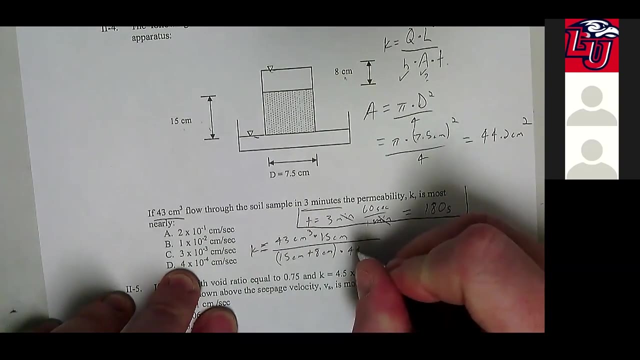 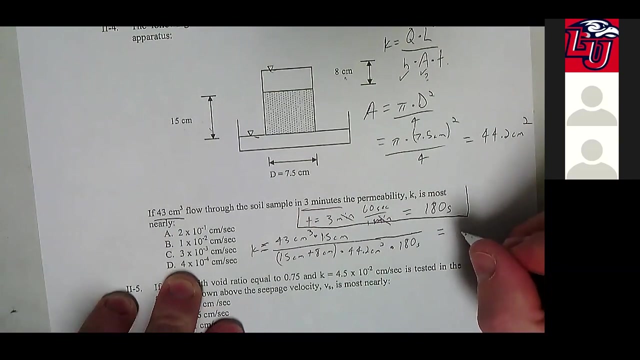 centimeters. Remember it's 15 plus 8.. Let's just write that out explicitly. Times area, which is 44.2 centimeters. squared times time, which is 180 seconds. Does anybody want to give me their answer first? 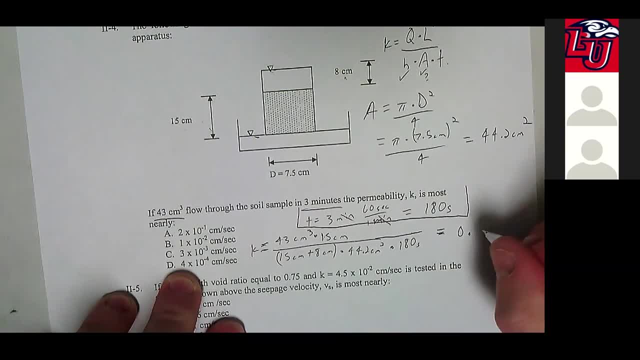 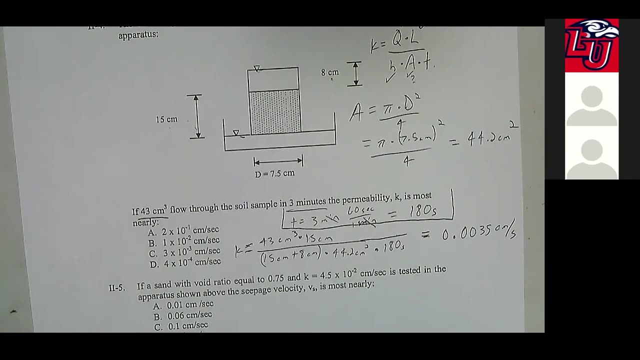 Everybody's fading after a long day. About .0035 centimeters per second. Anybody else get that number? Yeah, that's it Okay. So that's going to be closest to answer choice C. Okay, All right.